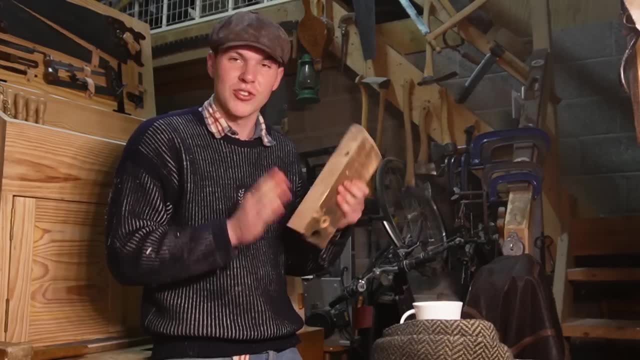 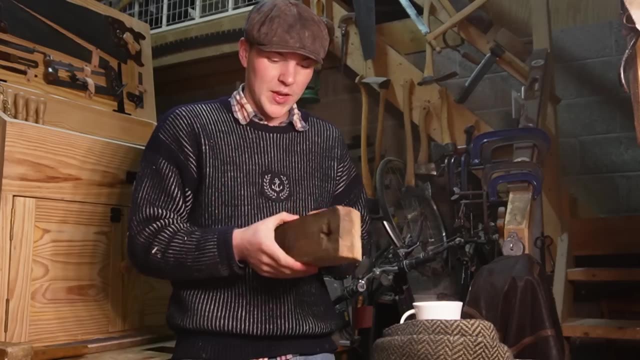 and I replaced the wood. but I hung on to this section of beech just because I thought I might use it for a mallet down the line. So it's been sitting in a pile of wood here for as long as I can remember. So today we're going to cut off all the excess bits on either side and get it ready. 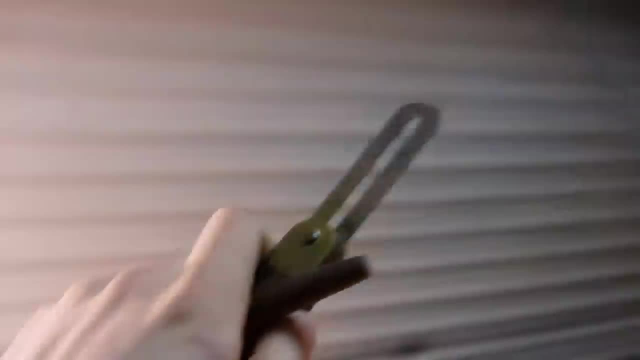 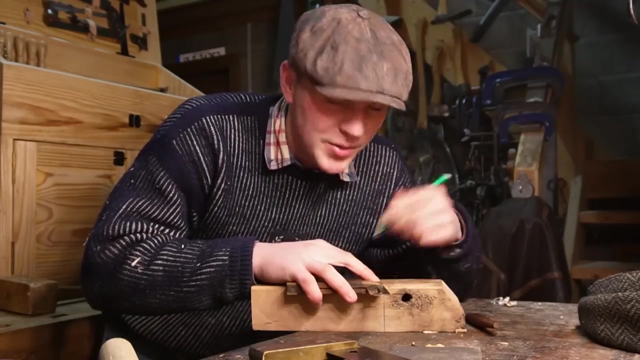 to go. I'm going to grab the marker knife and the sliding bevel gauge out from the box. here I've already got a square and now we're going to mark her out. So I oftentimes get comments with people asking what's the best beginner project and I always tell them: make yourself a nice little. 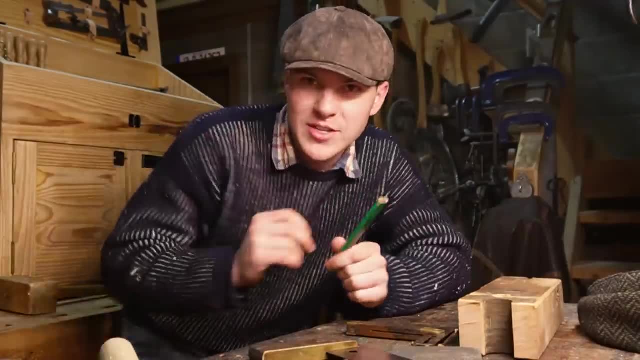 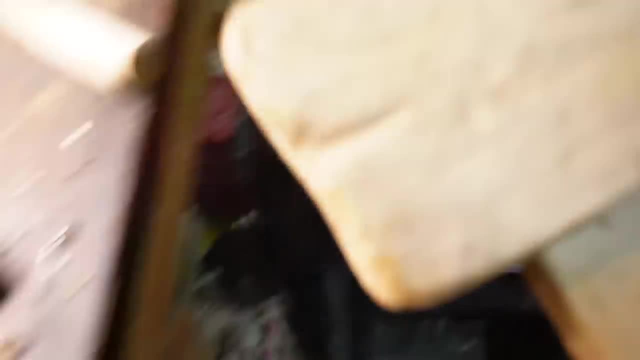 mallet. The first project I ever made was a mallet, and I'm fairly sure I still have it. Come down here to the drawer. there's a few more mallets, but this fella here, right on top, there it is. You can see my name stamped in there: 2020.. 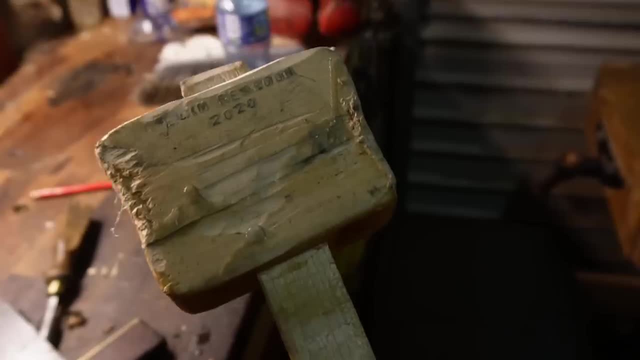 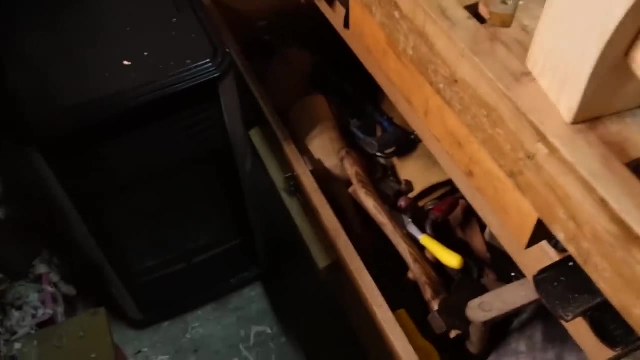 It's only two years ago. There we go. we can see it's fairly battered. I've had to glue it together a few times, and just a few days ago I made this beast of a fella here. So we've come quite a bit. 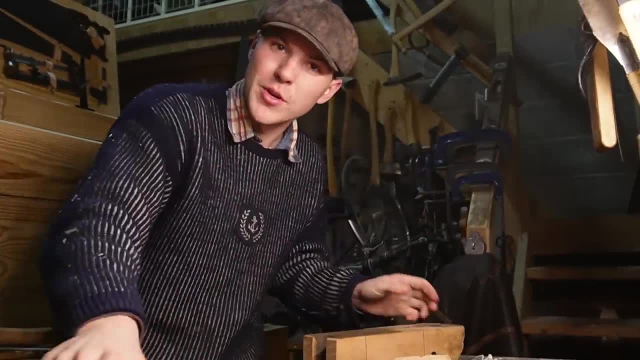 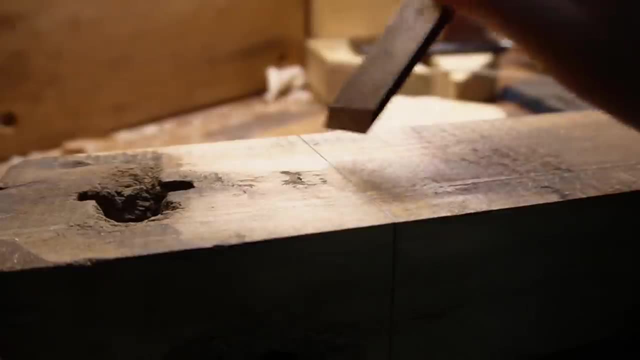 of a way. So I have it all marked out there now with the pencil. Now what I'm going to do is I'm going to come along with this chisel here and just mark out the line properly. So I'm just making sure the bevel of the chisel is facing away from the actual mallet here and I'm just 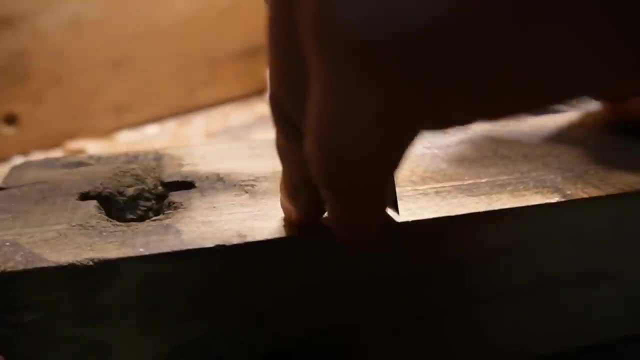 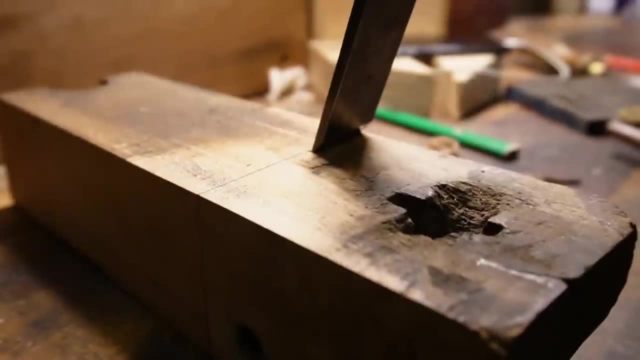 striking down like that, and I'm doing that the whole way along the line. So I'm just making sure the cut. So then I'm going to turn it around and this time I'm going to face the bevel towards the cut we just made and just give it a strike like that, and that should allow us to kind of peel a. 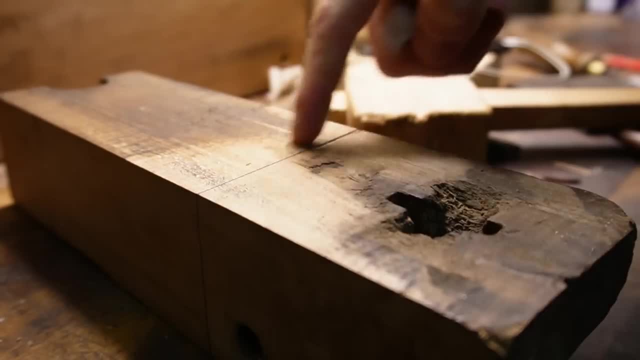 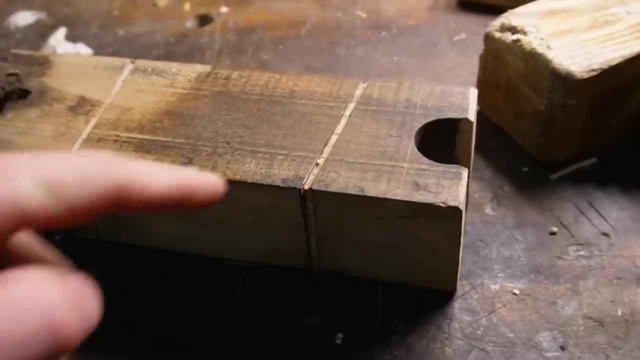 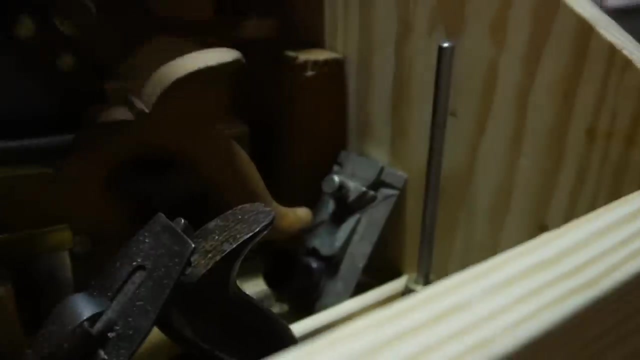 groove the whole way along our line and eventually, when we bring a saw to that line, this groove will help the saw kind of slide along exactly where we want it to go. So we can see there: now we have all these grooves cut down. Now we're going to go up and we're going to find this fella back here and 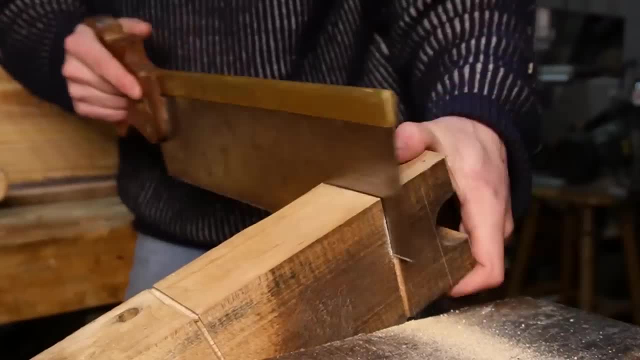 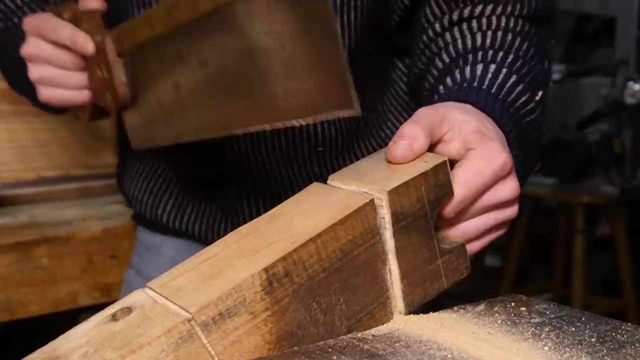 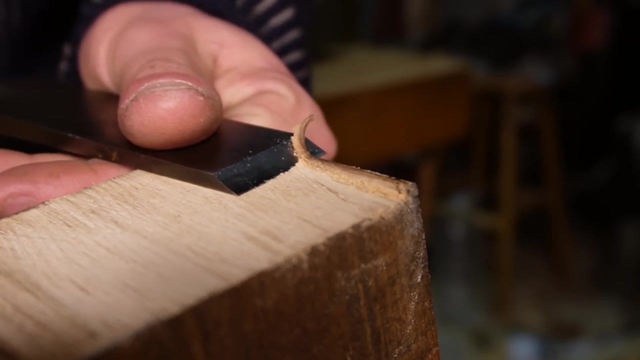 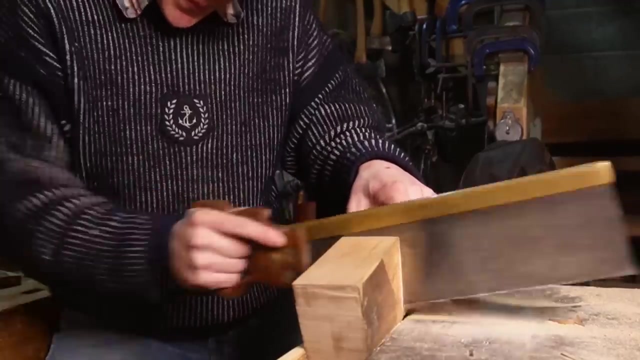 we're going to use him. There we go, just like that. There's a little bit left over here, so cue, satisfying chisel moment, There we go. Oh god, that took a bit off the side, but here I will manage. Here we have it. 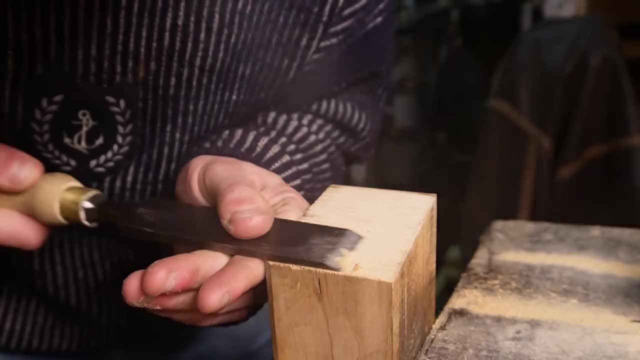 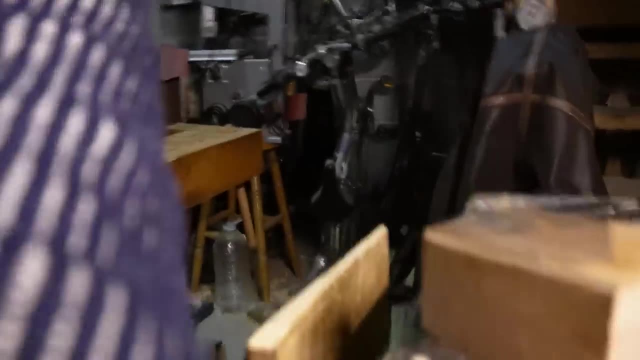 One more time. Once again, we're just going to come along with a chisel and clean that part off, So we can see there now all the growth rings in the grain. It's gorgeous, isn't it? So there's a bit of patina on it just because it's so old. So I'm going to chuck it into the vice here and grab the 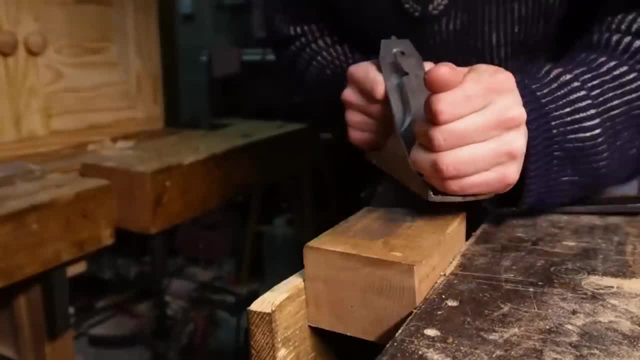 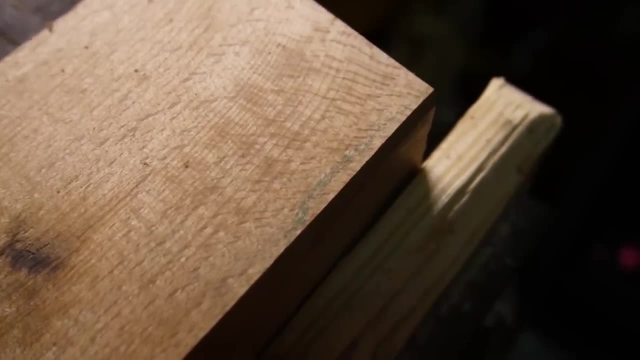 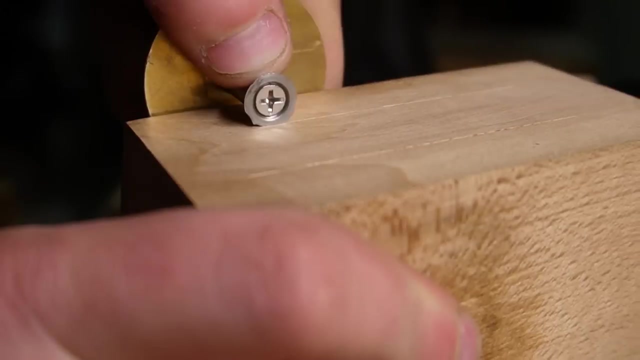 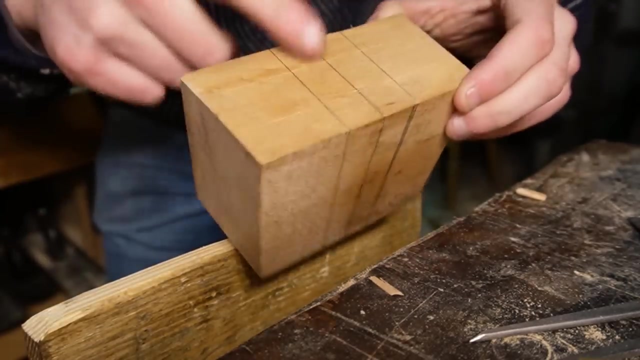 stallion number three and just shave all of that right off. That to me looks like a patch of green, however that happens. So I'm just using the marking gauge here to mark out the mortise that will eventually slot the handle through. So it's tapered so that the bottom is narrower than the top. so before I bore the hole the entire way through the mallet head, I'm 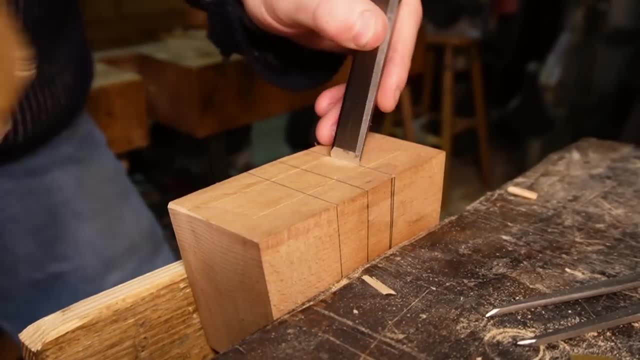 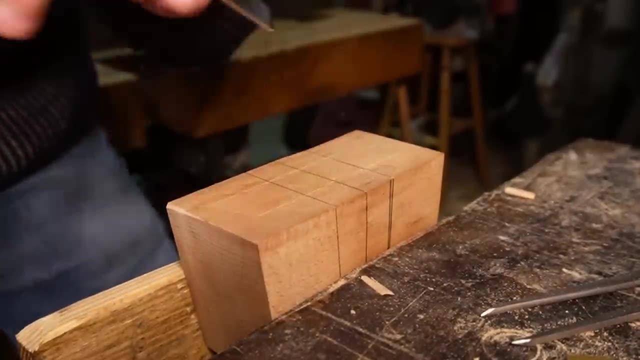 just going to come along with the chisel again and just mark out the shape of the mortise. That way when I do bring the bracing bit to it it wont tear out more than it needs to. so I will just spend a few minutes here. 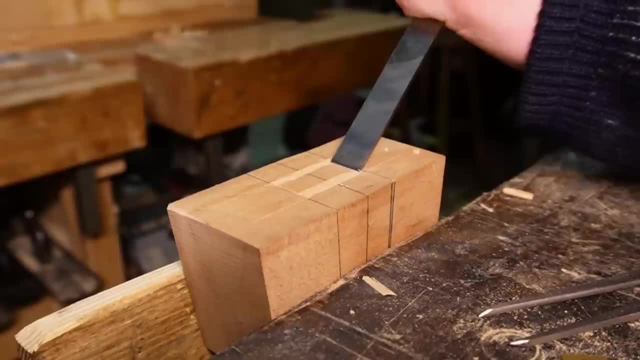 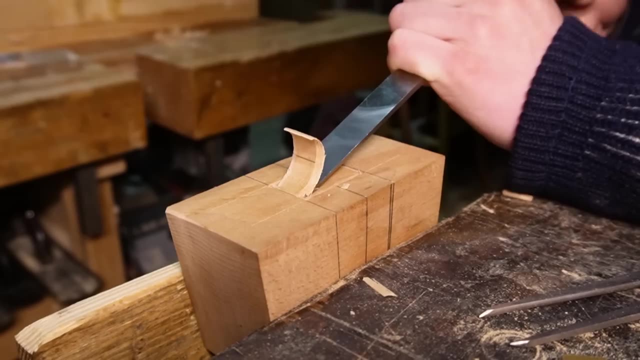 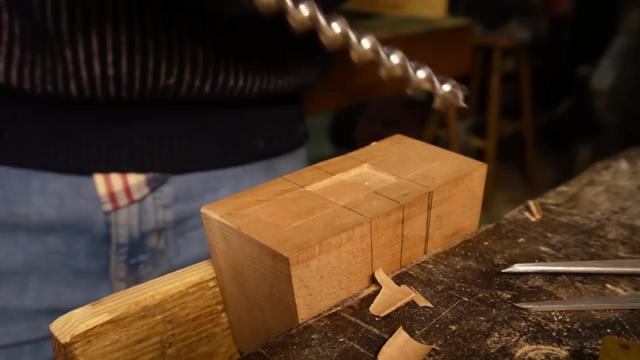 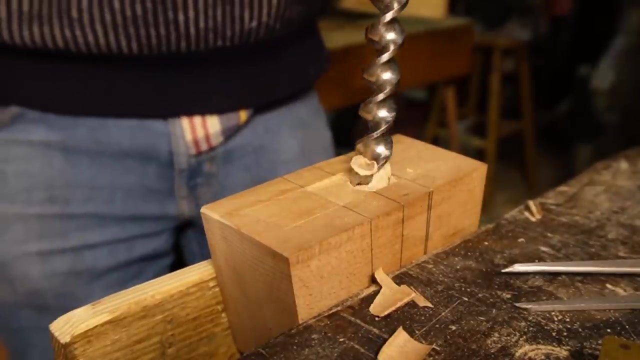 Tipping away with the mallet. So I have my bit here and my brace and I'm just going to screw it all together and use it to bore a hole the whole way along the mortise, and that will just allow us to remove all the excess wood a lot easier with the chisel afterwards, instead of doing the entire. 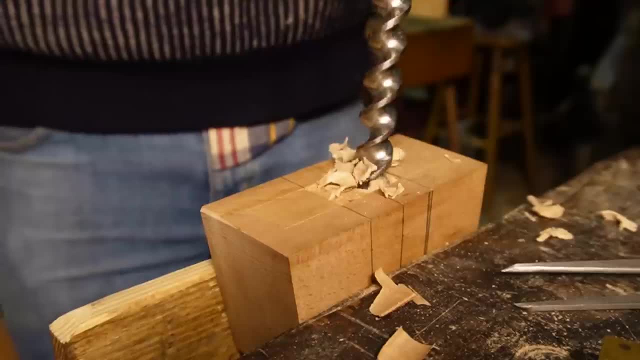 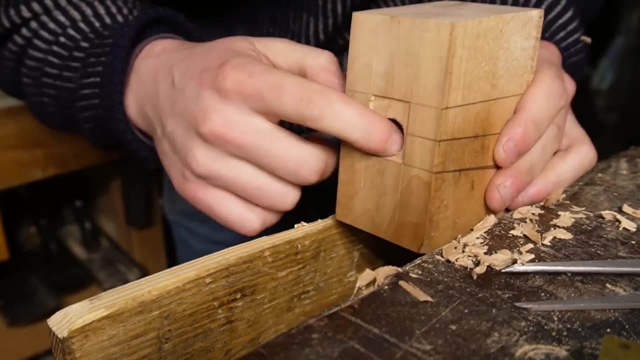 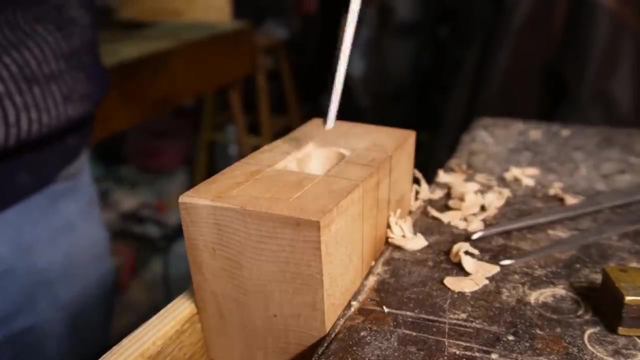 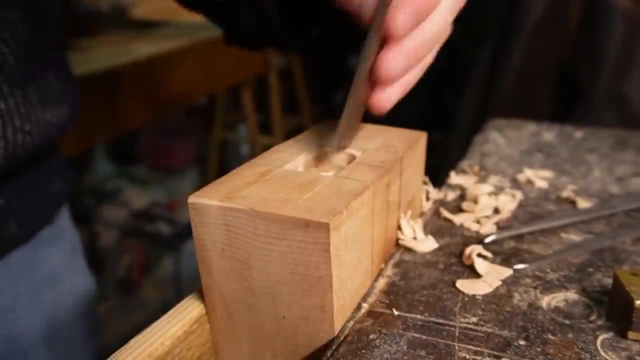 thing with just the chisel. We nearly missed, but we got that fairly close now. Then we can just come along with the chisel here and finish off what we started. Once we have the mortise bored, we have a perfect excuse to use this tiny bit. 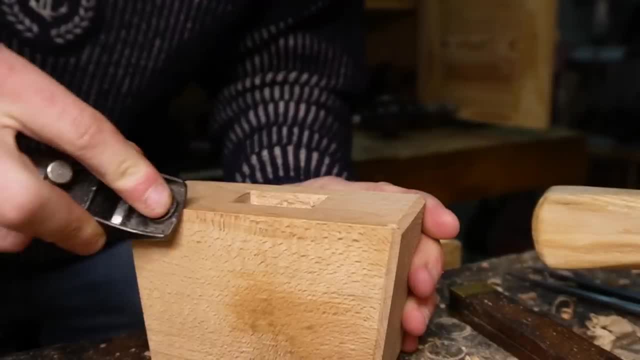 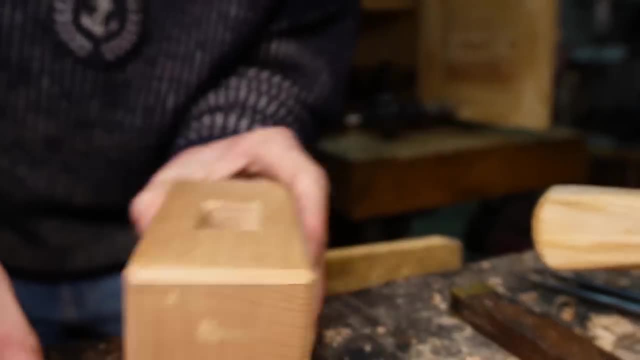 Tiny little Stanley 101 here just to cut the chamfers. so that's just a 45 degree cut on all the edges. we've already this side done and what that will do is it will lessen the likelihood of the edges getting battered and breaking out and splitting. so it's a very 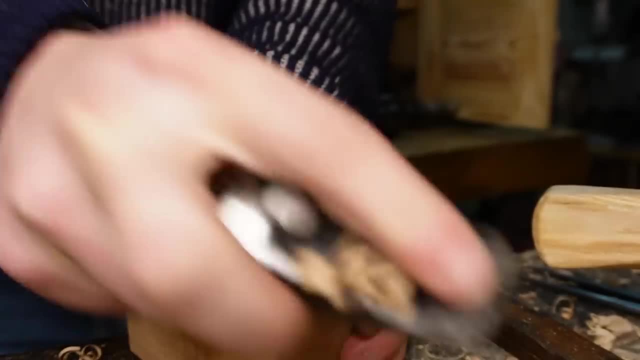 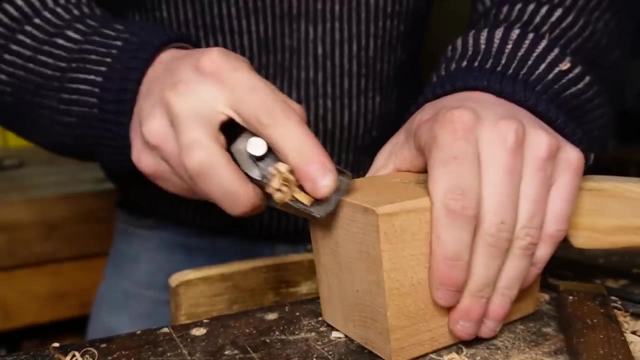 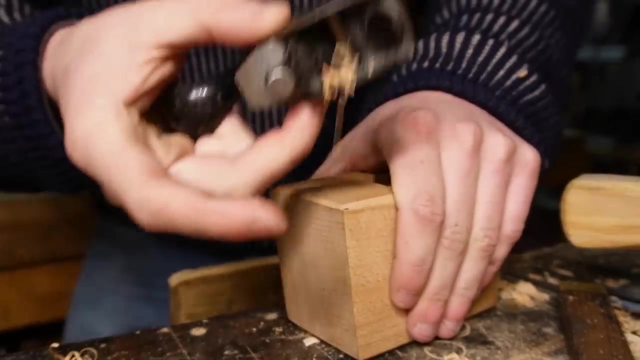 simple technique but very effective. You want to make sure you have a good sharp edge on that iron if you are going across the grain like this. You can see there now and it's good and sharp, It's nice and satisfying and we actually get ingrained shavings. 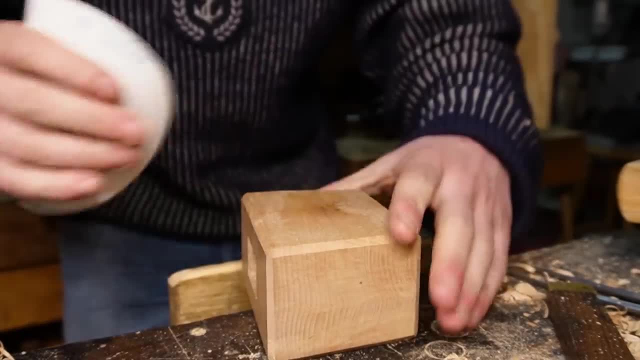 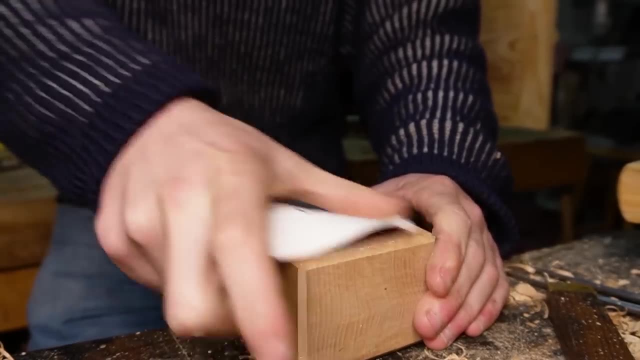 Now I could probably get away with just leaving a nice plain edge. but just because there's a small few patches of tear out here and there, I'm going to bring up some 240 grit sandpaper here and just give the whole thing a light sanding. 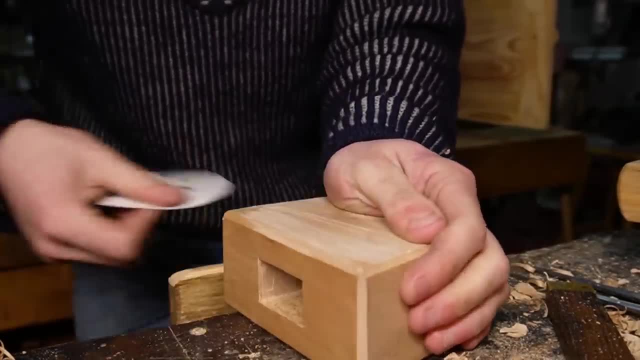 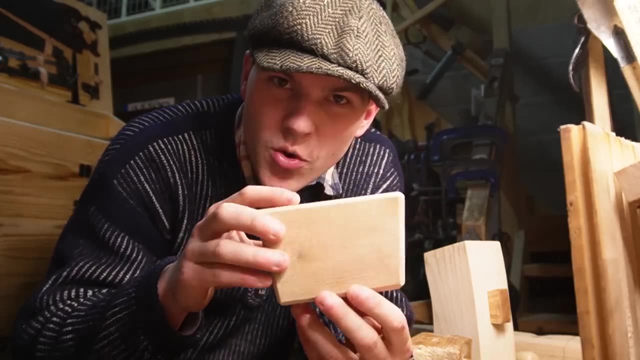 I kind of want to be gentle on the edges, don't I round them over too much. but that's what we'll do there now, and once we have that finished the head will be done and it will be time to move on to the handle. So I think I have the head pretty much ready to go now. 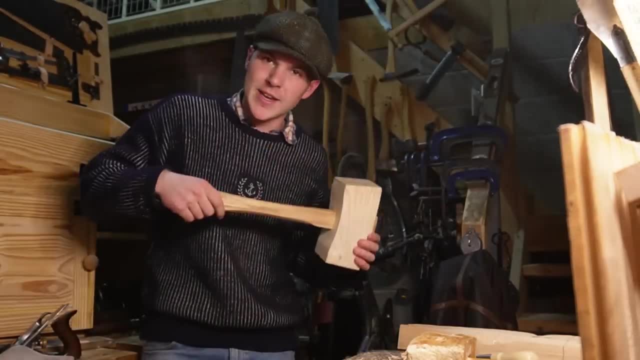 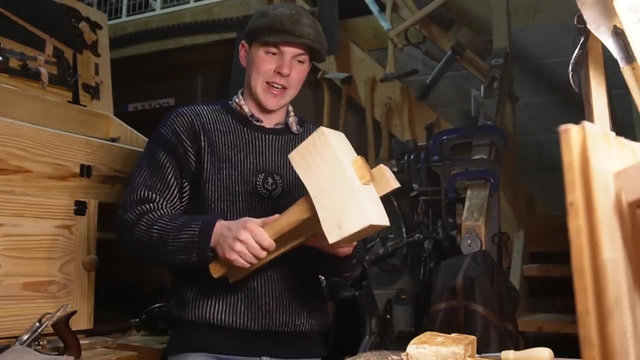 So I'm going to set the chisel down. I've got that behind me and it's time to start working on the handle. Now. I have a piece of ash left over- the same piece of ash I used to make this handle. so it's a bit too long now just because I needed a longer handle for this part, but I'm going. 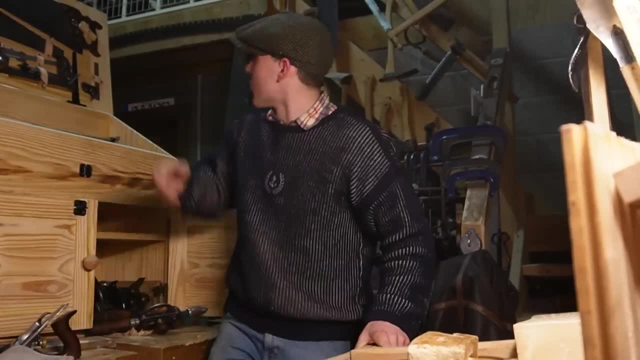 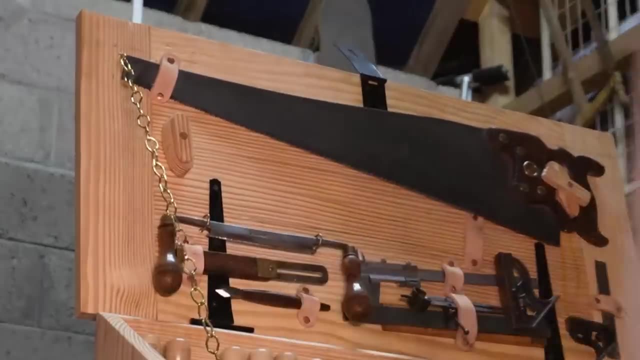 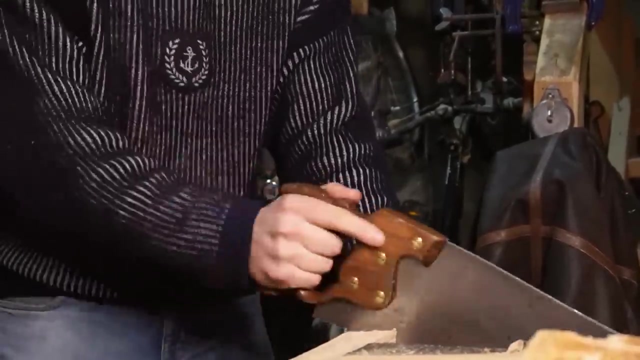 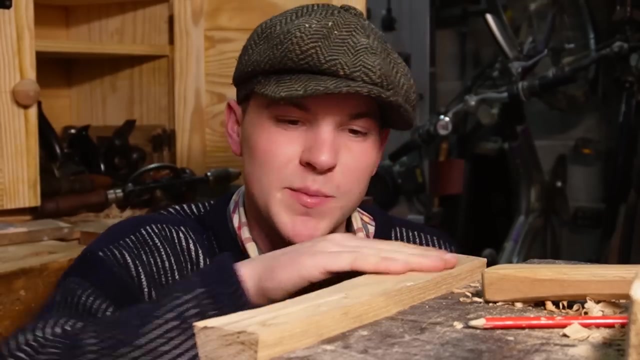 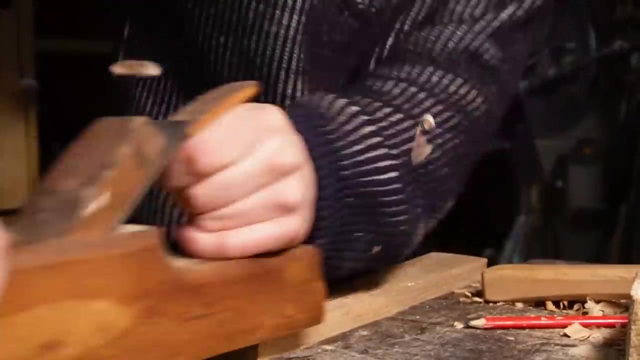 to throw it in the vise here and pull out our rip cut saw from above here. So I have it in my vise now and the first thing I'm going to do is make this completely flat and true and then I can worry about getting the shape of the handle later. 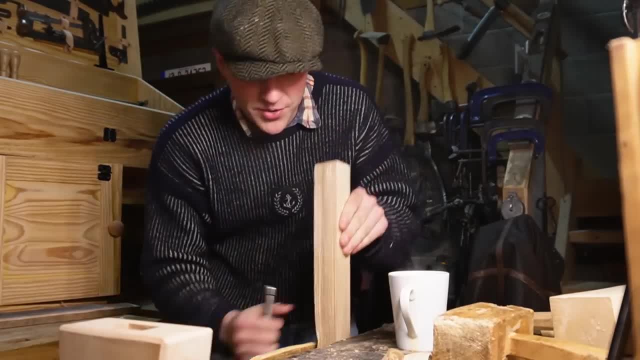 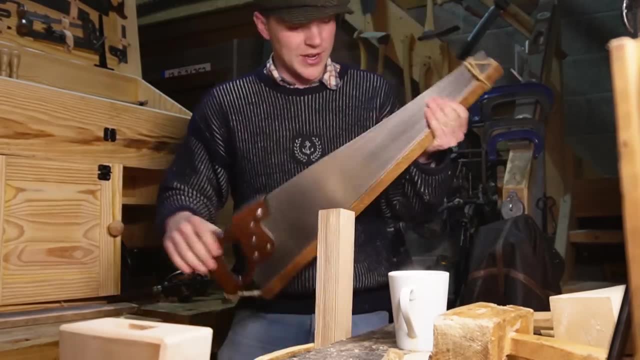 So the rip cut saw in the box isn't sharp enough and I don't have a triangular file because the one I do have is broken and the shop that I buy them off doesn't have it in stock. But I do have one rip cut saw right here, this Diston that I know has good, sharp teeth. 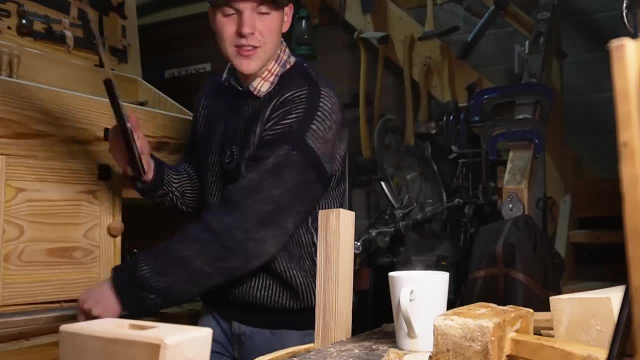 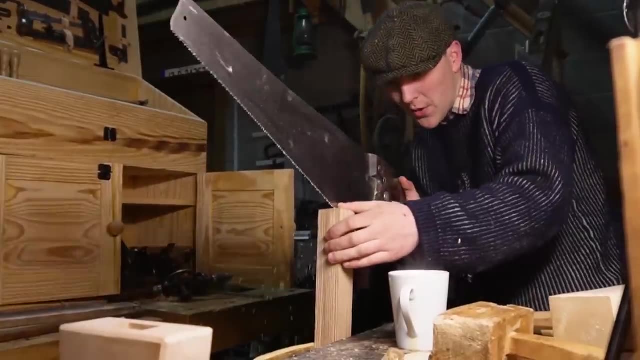 on it because I make sure to put the guard on them every night, or the sheath, or whatever it's called. So we have it locked in the vise there now and I'm just going to spend a few minutes ripping that down along the length. 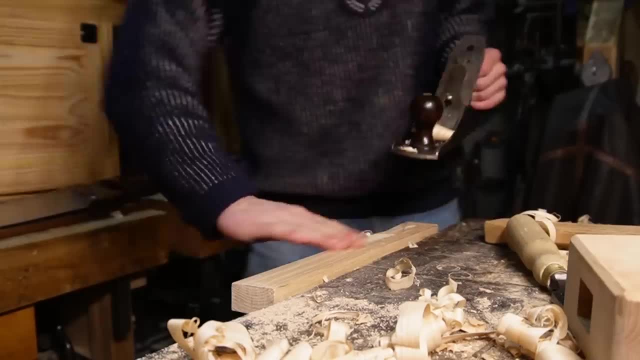 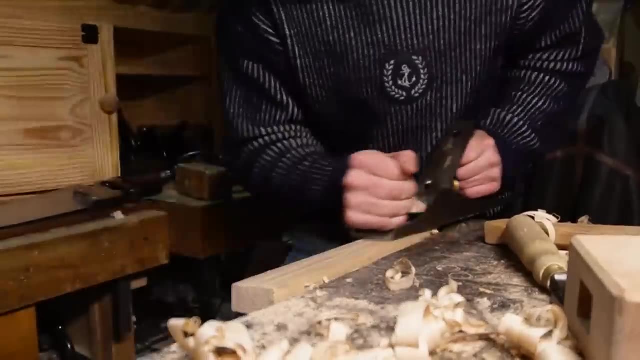 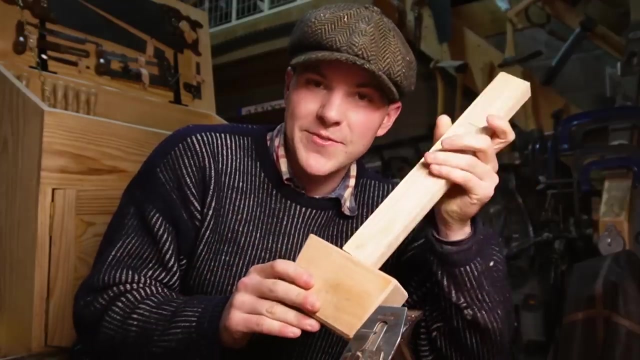 So just to get the last side smooth, here I have the number 5 that I'm just kind of planing it down with. Alright, So in order for the handle to fit, it needs to match the taper. basically, the mortise is wider on top than it is on the bottom, so it should just slot into place. 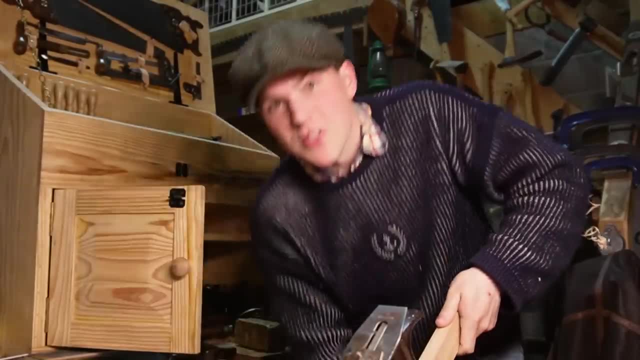 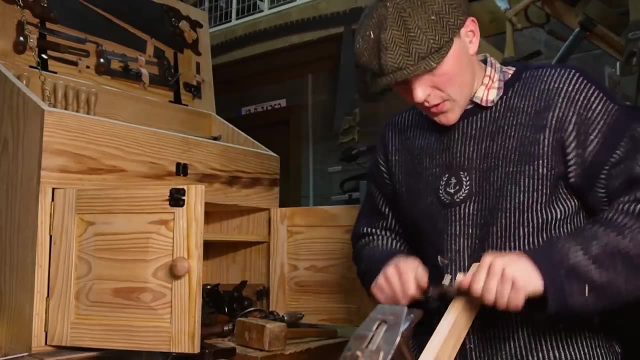 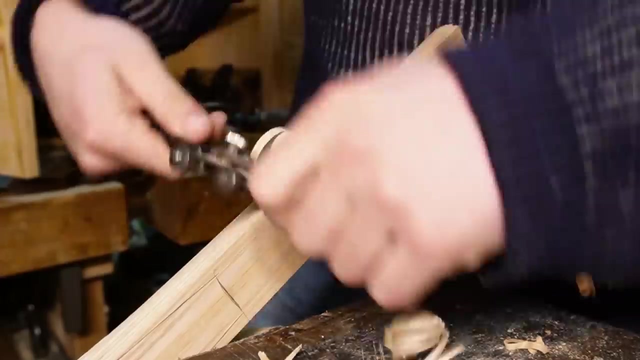 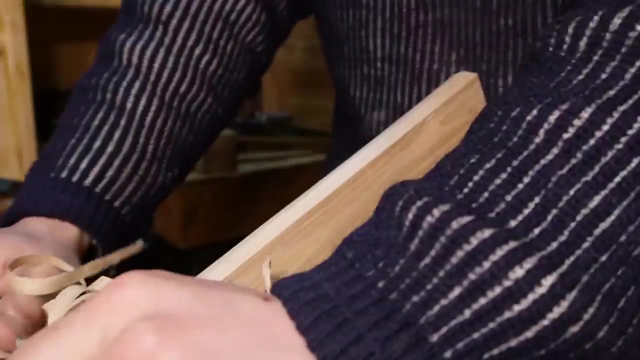 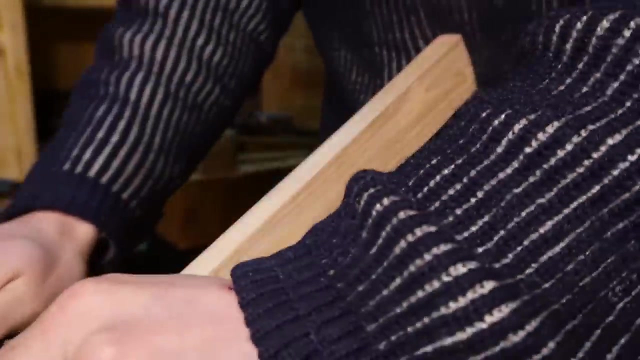 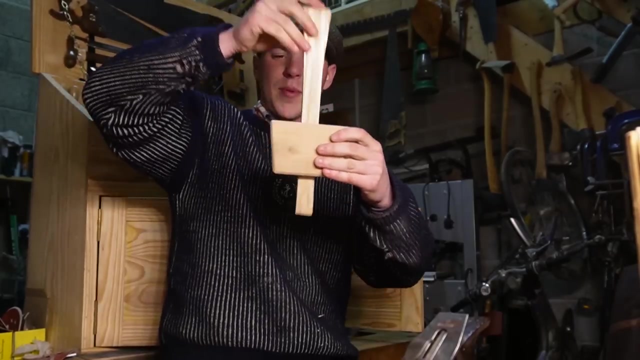 So, in order to get that taper on the handle, I'm just going to throw it into the vise here, grab my spoke shave and just work my way up like this: Alright, Alright, Alright, So, just like that, Right. so, moment of truth, we have the thing tapered and we're just going to drop it in. 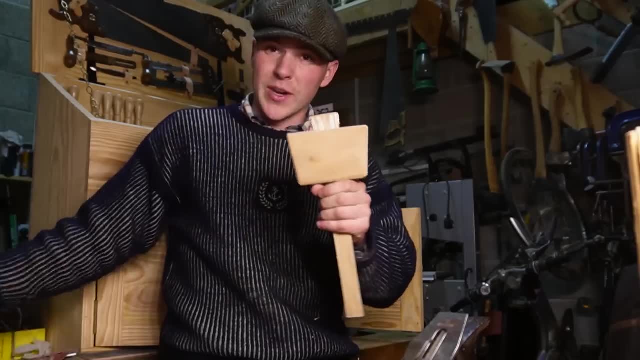 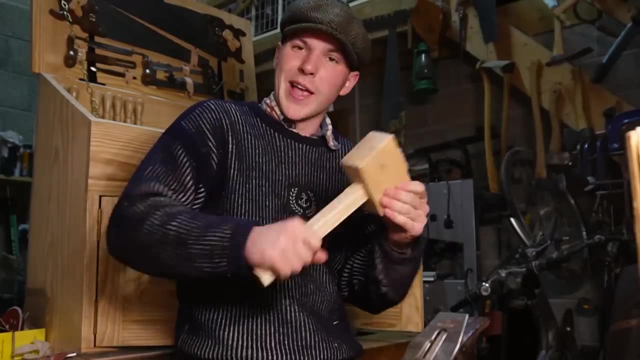 like that. See how far we can bring it with our hands before getting the mallet and just locking it into place. There we go. So we need to round out the handle, But it feels fairly good and very lightweight, which is kind of what you want, nothing like. 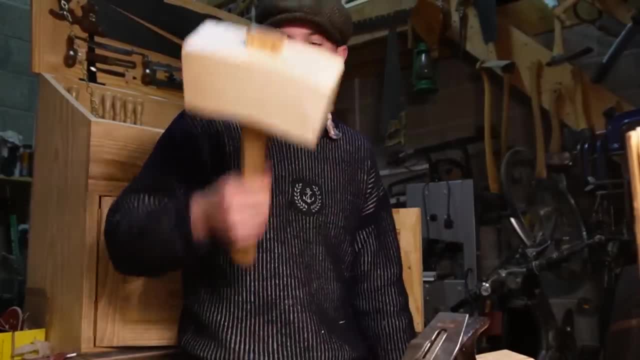 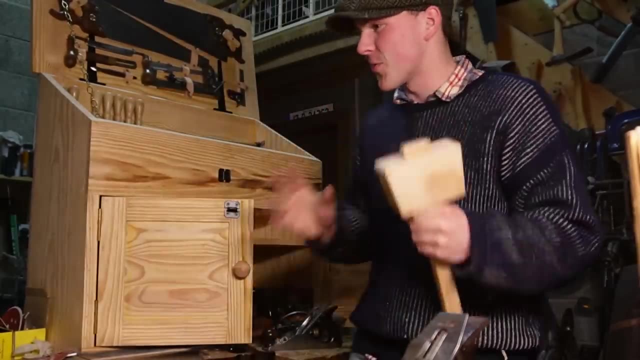 this monstrosity, just totally. yeah, this is a novelty item, in fairness, but no, I can see myself using that to step up from it. If I can find the first one I made, I'd love to compare and contrast because they're very 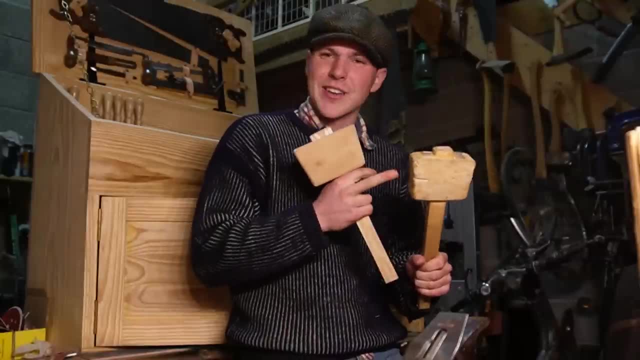 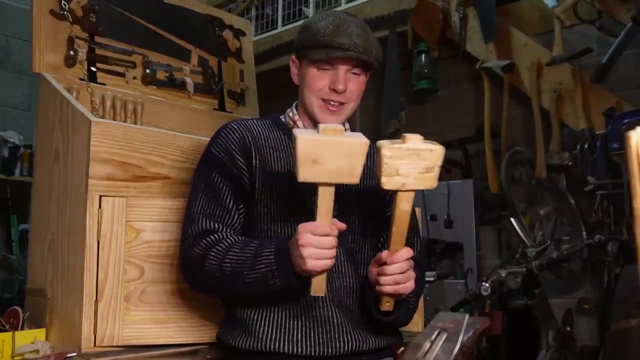 similar in design. There we go. I remember this was actually a second or third attempt before I finally got something looking like this, But this fella now is looking a bit more square and clean and even so, In a mad watt, In a mad watt. 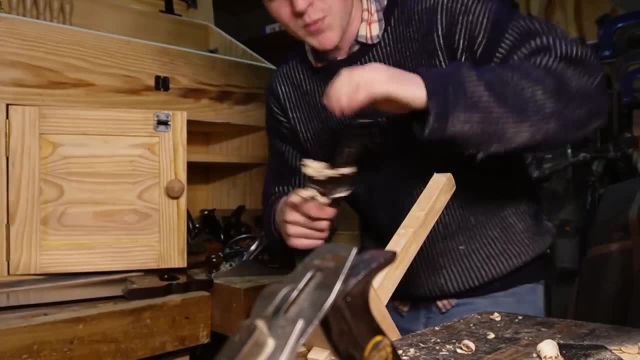 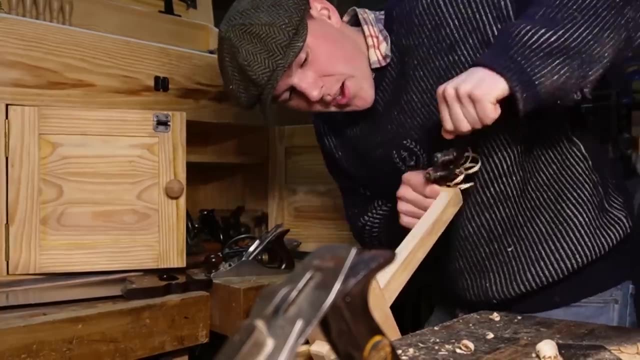 Just over two years, can do. So. to round out the handle, I'm just going to take the spoke shave and I'm going to count how many times I go on each side. so I'll do three, four, five, six. So I've done six on that side now. so I'll just repeat on this side and I'll do that.